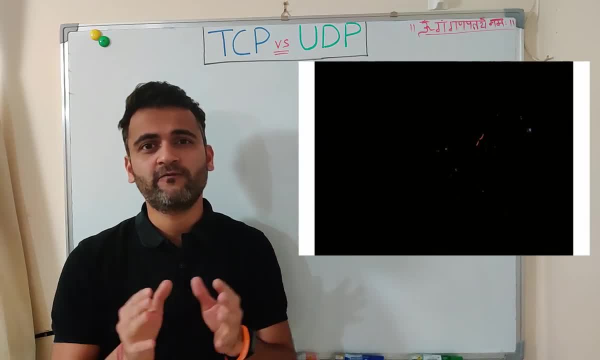 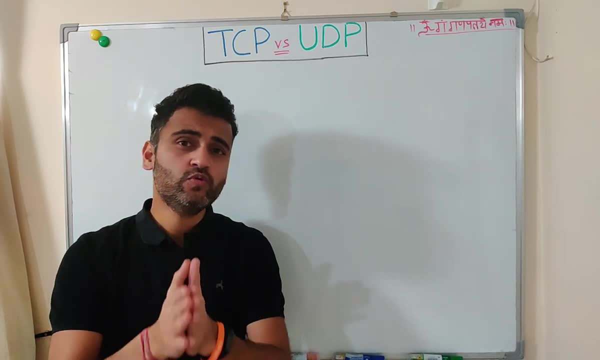 time and just right at that moment the electricity goes off and you are shattered. But within 5 minutes the power comes back up and you are jumping with joy. But hold on. would you want to watch those 5 minutes which are lost or would you want to exactly directly go live? 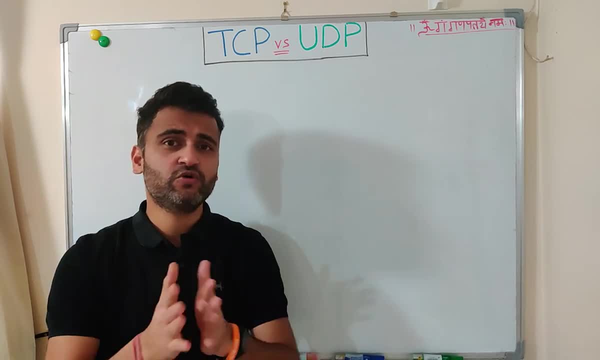 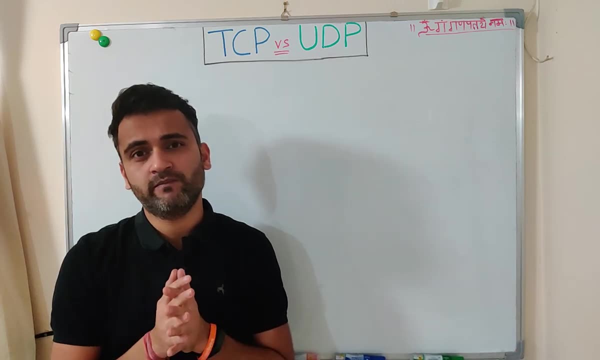 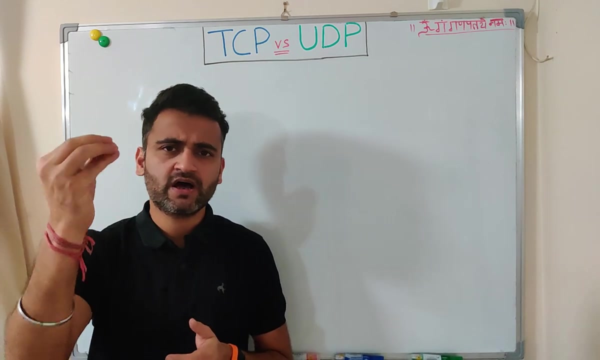 and see the match as it is happening. I am pretty sure your answer would be to go live as soon as possible so that you don't miss anything which is happening live on the match field. But now take another different scenario. Suppose you are shopping and you are buying some stuff. 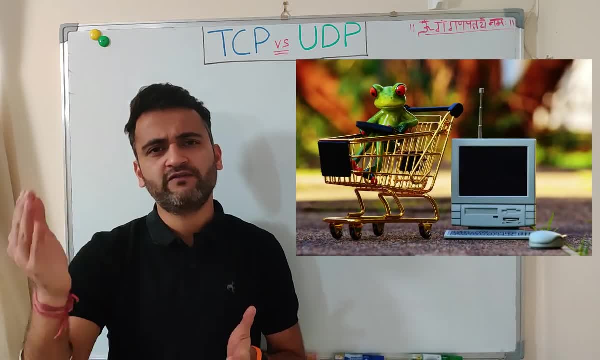 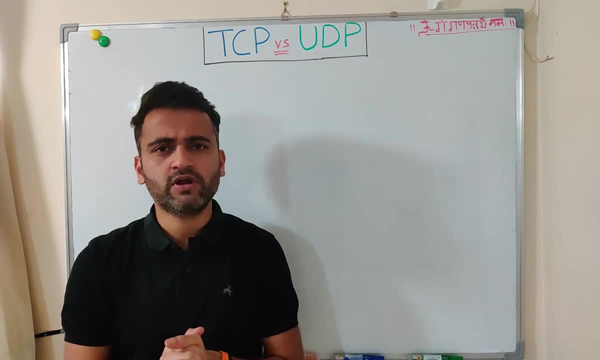 on an online portal- online e-commerce portal- and you have added that particular product into the cart and you are now proceeding towards checkout. and during the checkout you observe that while doing the checkout directly, the payment page comes up, but the portal did not ask for your address and you made the payment. 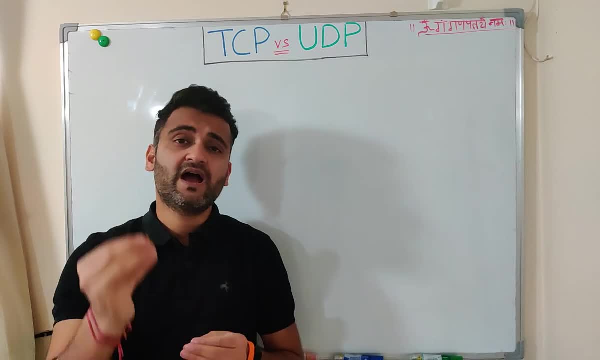 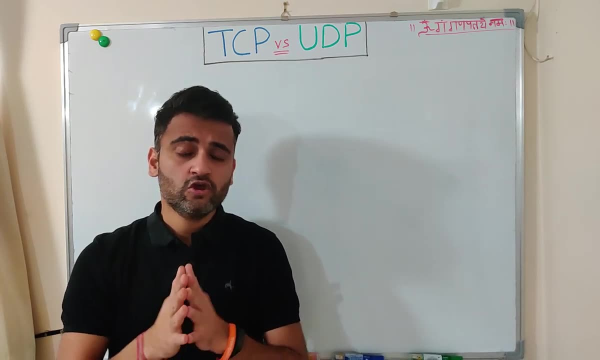 Would you want that to happen? No, You would always want that your address is taken first and then only a kind of payment can be made for that particular product. So there are two scenarios. One is a soccer match, where you want to see the live match. 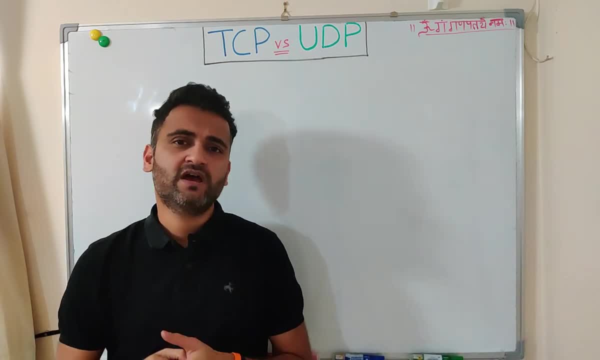 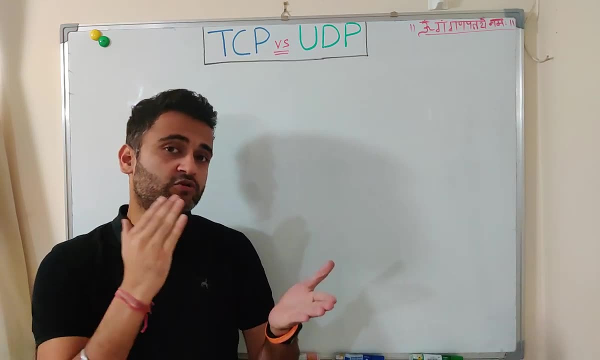 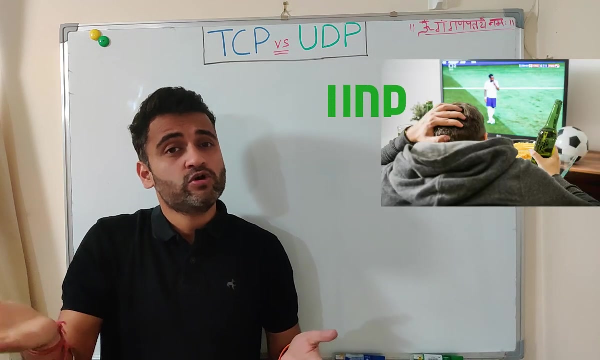 at speed and directly, exactly without any interruption, wherein, here, while you are buying a product, You want more reliability as to you should not be, you know, messing up with your payment and your address and everything. So your live soccer match can be correlated with UDP and your reliable online portal ordering. 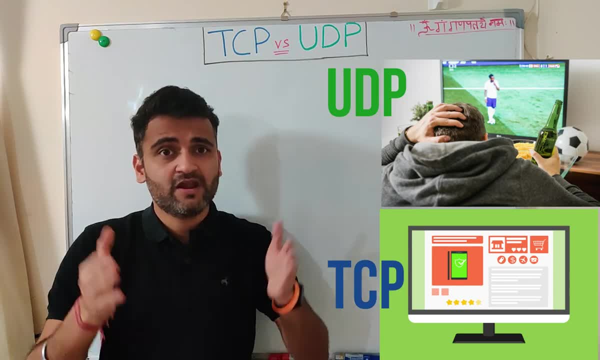 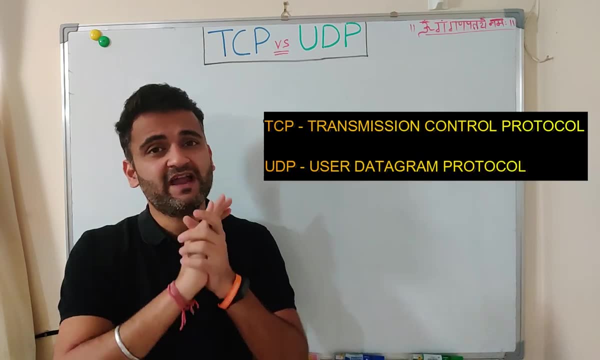 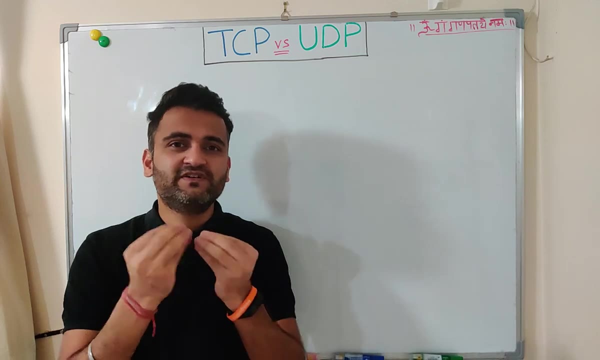 system can be compared with TCP. Now let's understand what is TCP and UDP. As the name suggests, TCP is transmission control protocol and UDP is user datagram protocol. Both are Based on top of the basic protocol, which is IP protocol, and are used to transfer information. 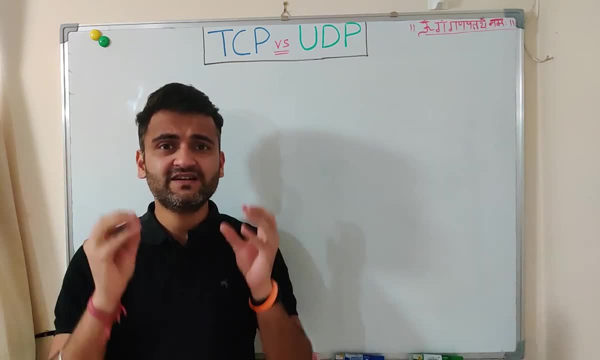 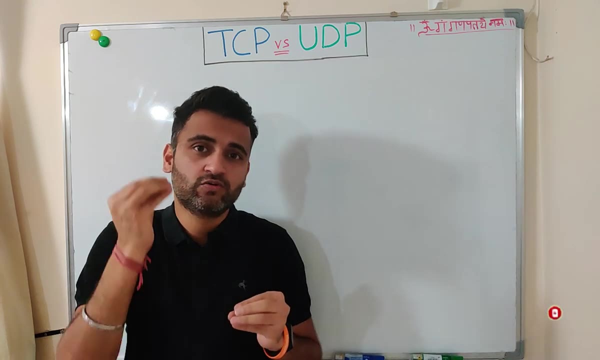 in the network from one device to another. But there are certain differences in which TCP operates and UDP operates and both have its own uniqueness, goods and the bads, And that's why, when you are deploying any kind of networking solution, you have to understand. 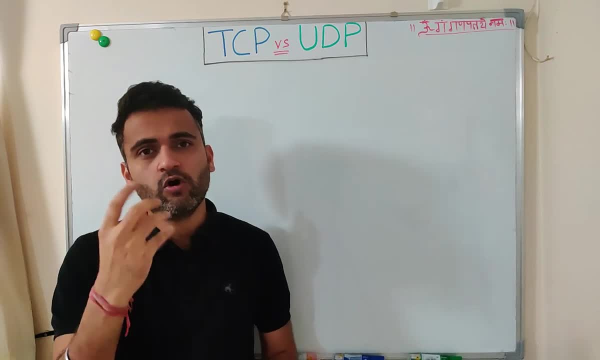 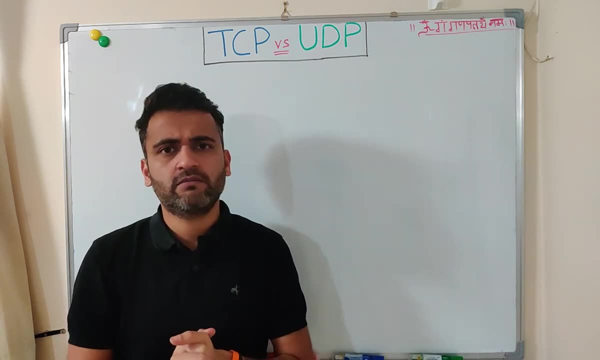 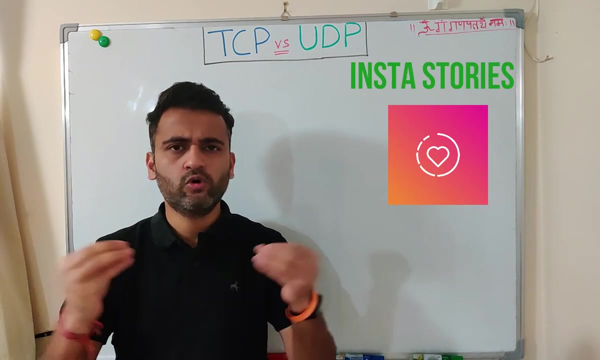 for your particular use case, whether a TCP is more suitable or a UDP. Let's take another example to understand it better. Suppose you have made an Instagram story and you put it into your Instagram account. You put it for all the whole of the world. 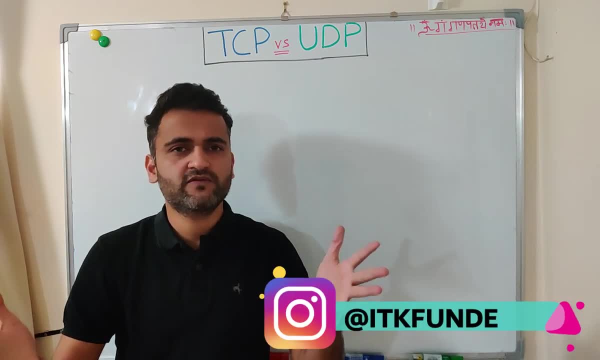 You are not bothered about who's seeing it, who's not seeing it. It will be there for the next 24 hours and then it will go away. But on the flip side, when you do an Instagram DM to a particular person, you are very, very. 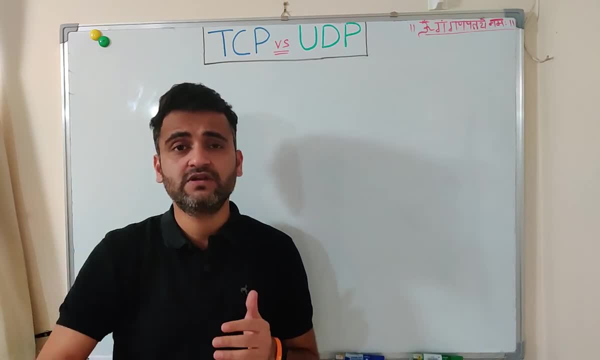 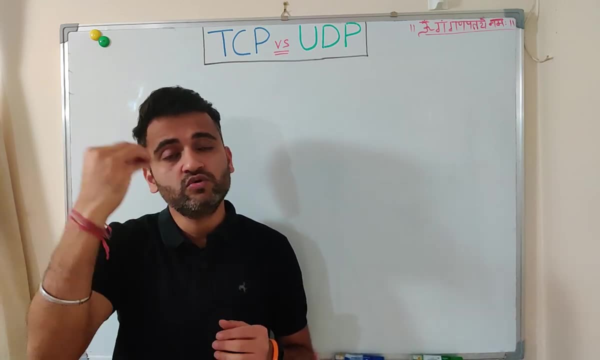 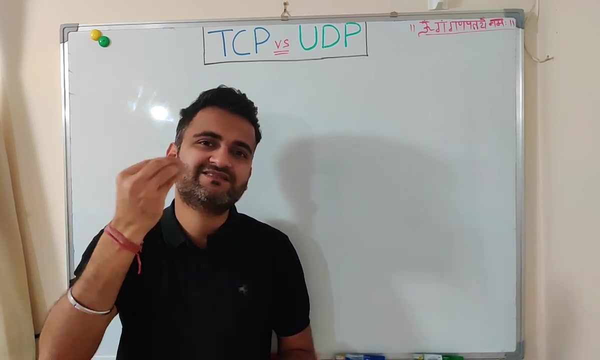 connection oriented. You want to make a one to one connection with that person. You want that person to reciprocate to your message and there has to be a two way communication between you and the receiver. Again, in a similar way, a transmission control protocol is something which is your Instagram. 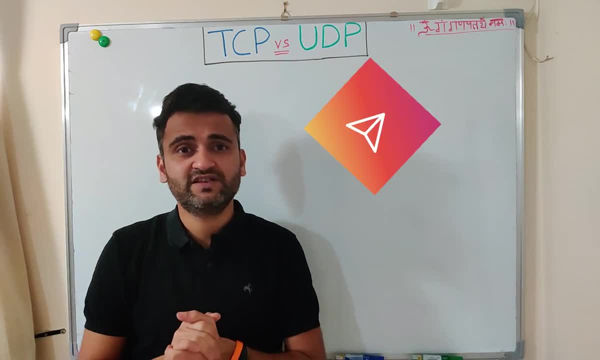 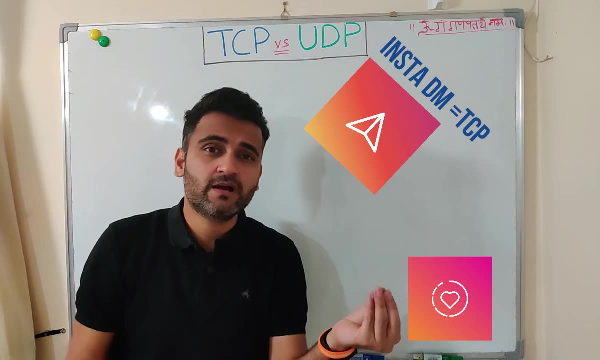 DM, where you are creating one to one connection with the sender and the receiver. There is a handshake, There is an acknowledgement On the flip side, on user datagram protocol is like your Instagram stories: You just broadcast it to the whole world. 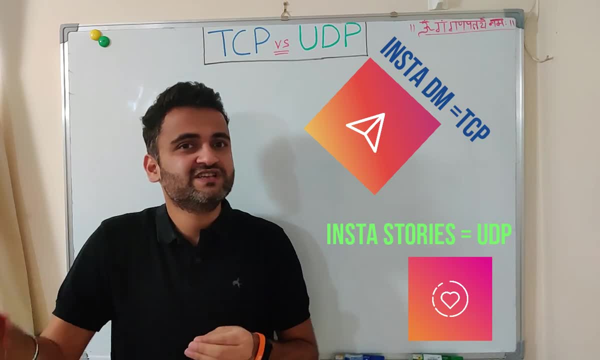 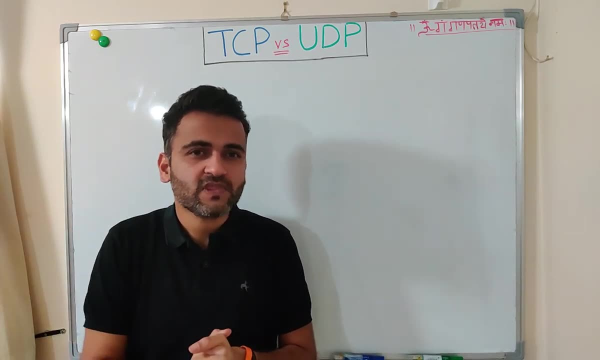 And you don't care that much about who's seeing it, who's getting it, who's not getting it. You just post it all and you just assume that whosoever wants to receive it would receive it. So I'm sure by these two examples you are pretty much clear about what is a TCP and 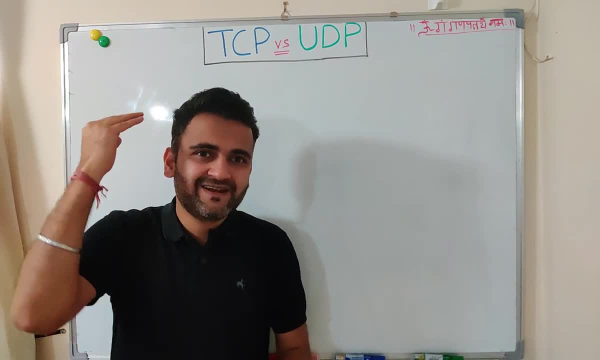 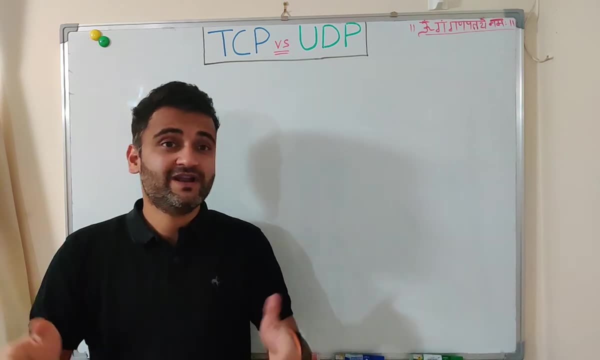 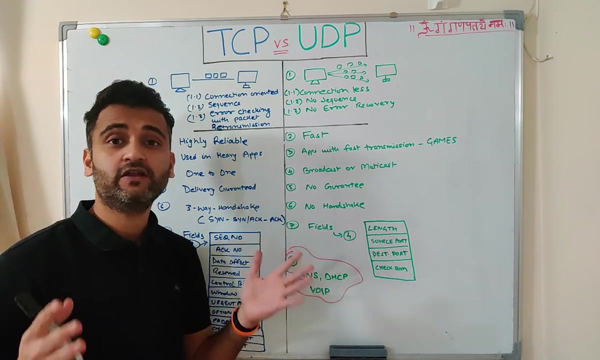 what is a UDP protocols. But now what we will do. we will create a left and right comparison between the two and go into the subtle differences these two protocol has. So let's go to the board and see those differences, Friends. Let's do some left and right comparison between TCP and UDP protocol. 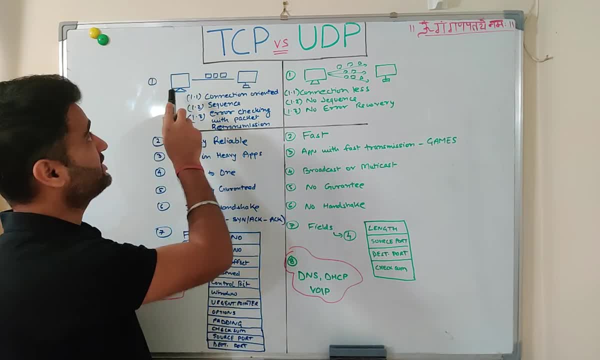 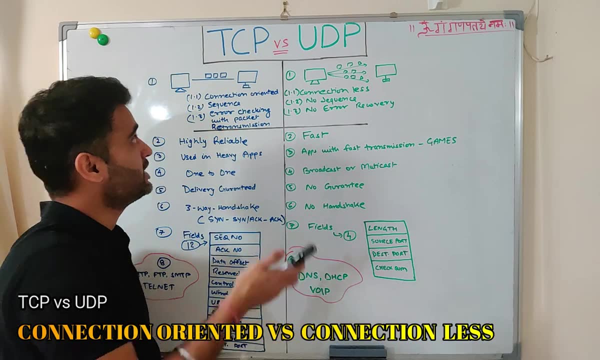 So at the first, as you can see I have drawn out in this diagram, TCP is very much connection oriented, wherein in here a UDP protocol is very, very connection less. What it does mean is that when a TCP protocol sends a packet over the network from source, 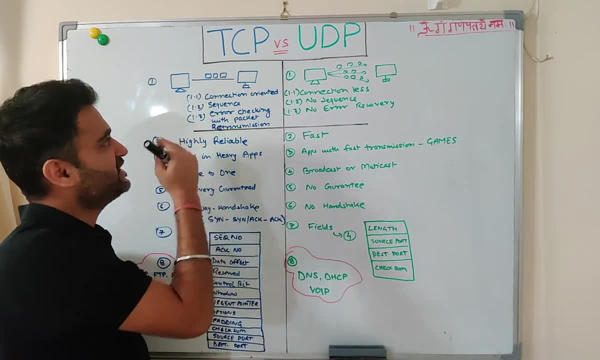 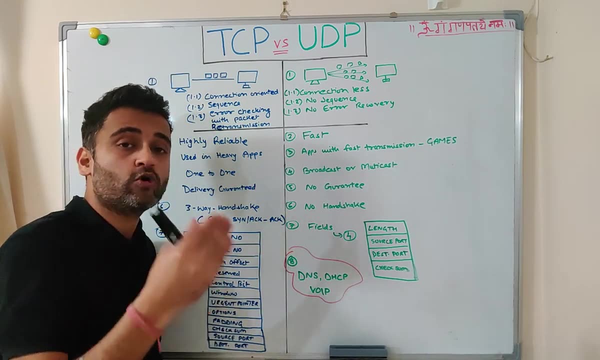 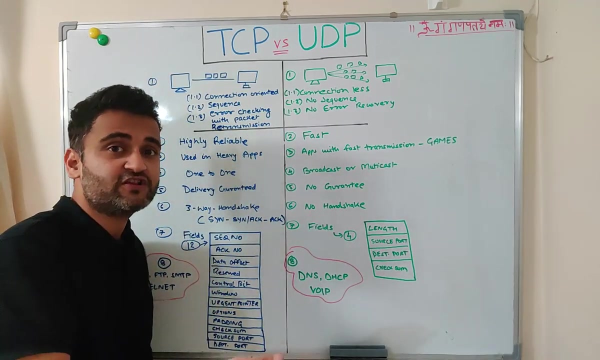 to destination. it follows a certain sequence and it follows error check in very rigorously to ensure that the packet reaches correctly, and then only the second or the subsequent packets are being sent. in case there is an error, there is a possibility of retransmitting the packet again. 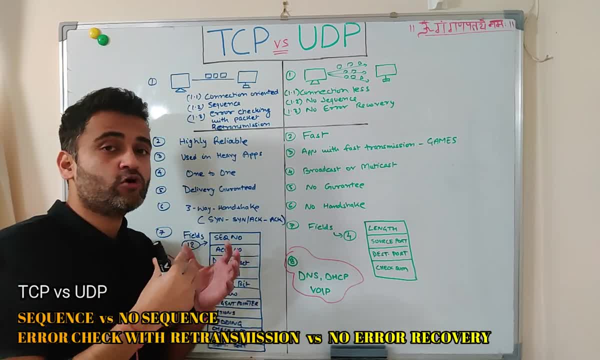 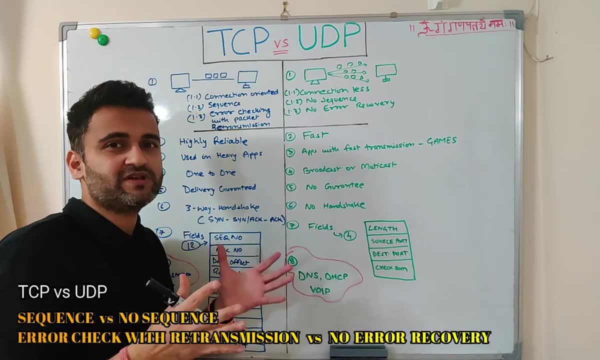 if the one particular packet has not yet reached successfully, tcp protocol will again resend that packet, wherein this particular, in this particular udp case, it is very, very connection less. there is no sequence in this and there is no error recovery. it's just that you just broadcast these messages. 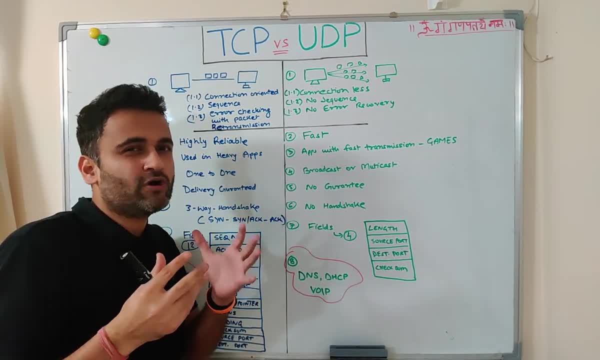 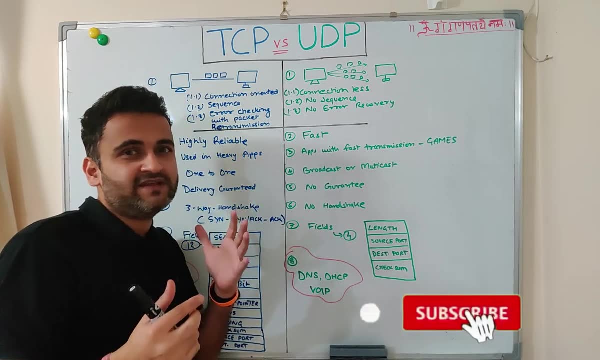 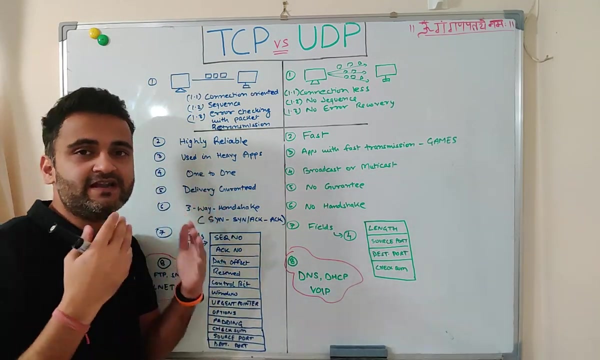 to the, you know, to the center, and udp protocol does not much care if some packets are lost or some packets reaches in wrong sequence. so basically udp. that's why is very, very fast, because it does not take care of these many things what tcp does. secondly, as we have already, 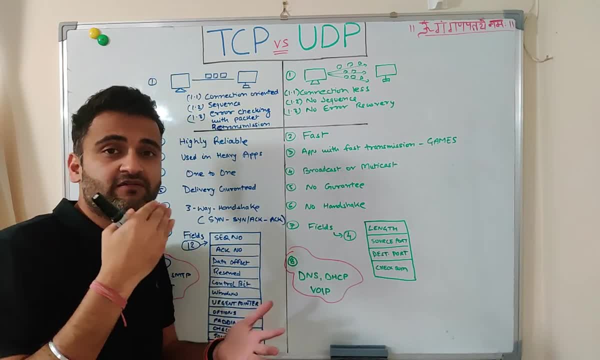 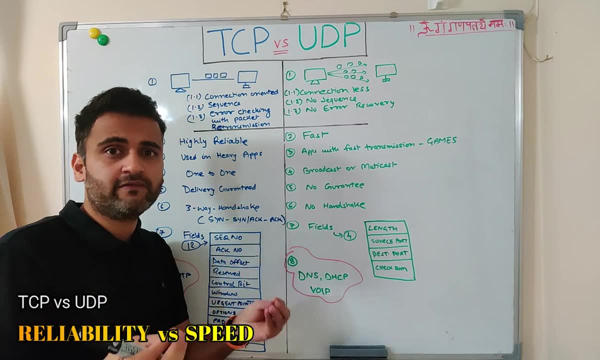 discussed couple of times, tcp protocol is very, very reliable, very, very secure and that's why most of the applications which needs security, which needs higher reliability, will always go for a tcp protocol wherein udp protocol are very, very fast for for transmission of packets. if you want to do it, suppose you are doing a live streaming or you are watching a 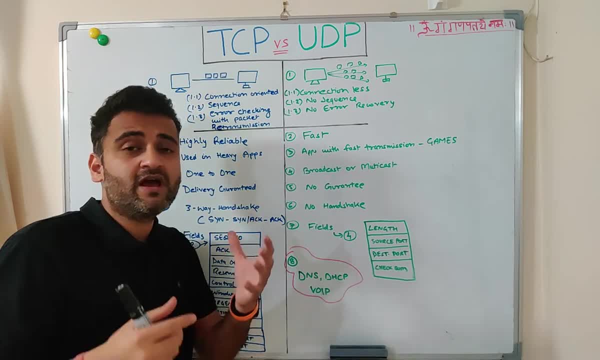 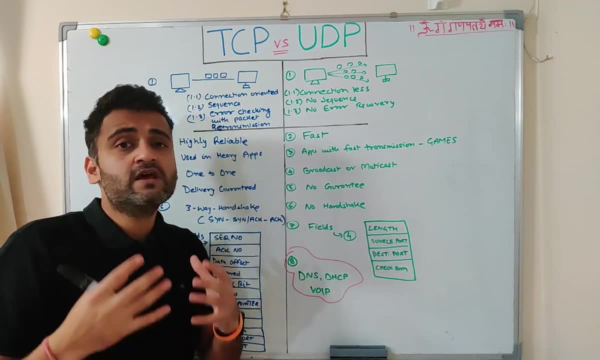 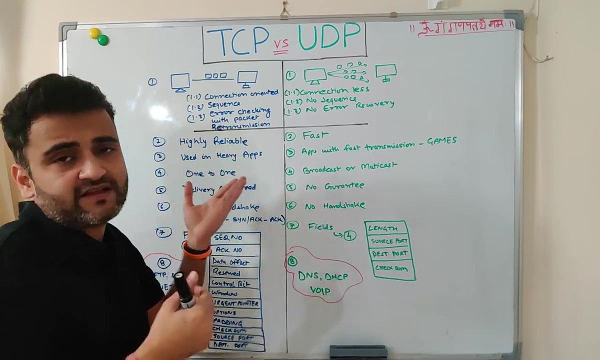 match, or you are using some online games or something. these kind of the scenarios, you know, the delivery is should the speed is the need of the rather than the reliability. that's why, in those cases, udp protocol is is preferred. thirdly, it is, as i said, used in heavy applications, which you know which needs resilience and which needs fault. 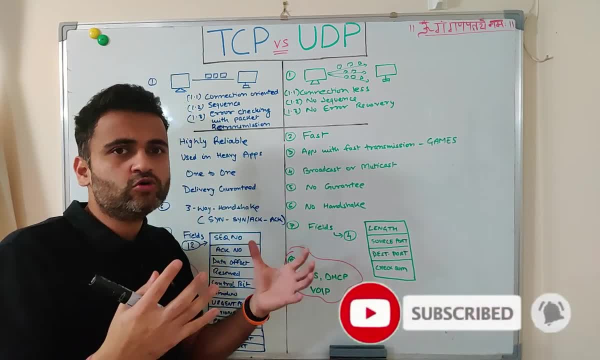 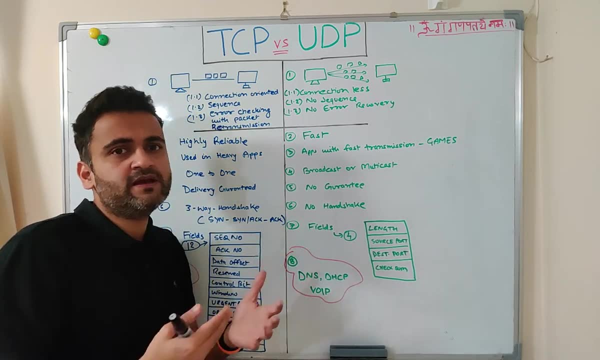 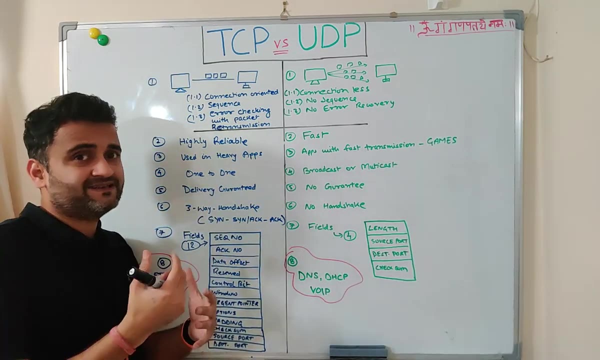 tolerance and which also needs security. in all those cases, tcp protocol is preferred and, as i said, for faster transmission like online gaming and things like that, applications like that- you will go for udp protocol. again, one-to-one connection is always there between tcp, between sender and the receiver, while they are using tcp protocol. tcp protocol. 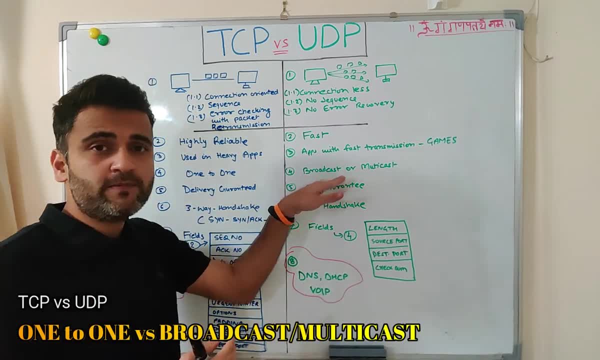 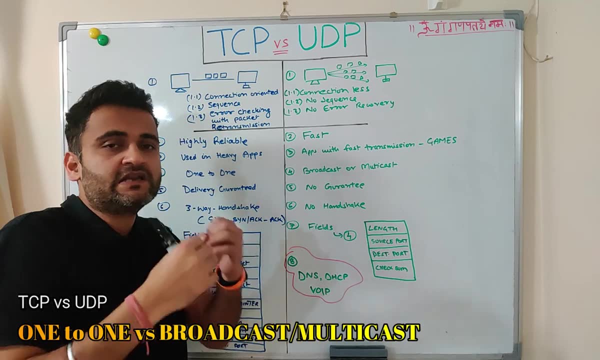 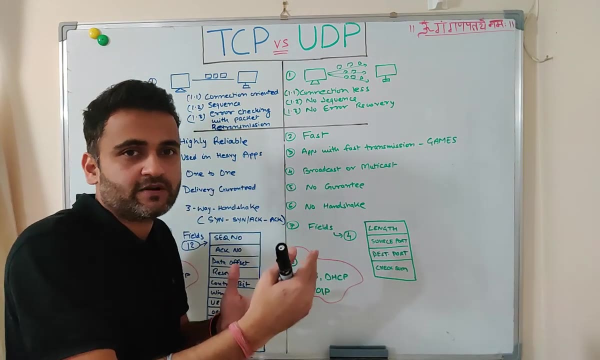 does not broadcast the message, wherein a udp protocol always broadcasts the message or multicast the message, like what we do in instagram or facebook stories. we put it and we let everyone know that we have put up a story wherein, you know, tcp is like a personal facebook messenger. 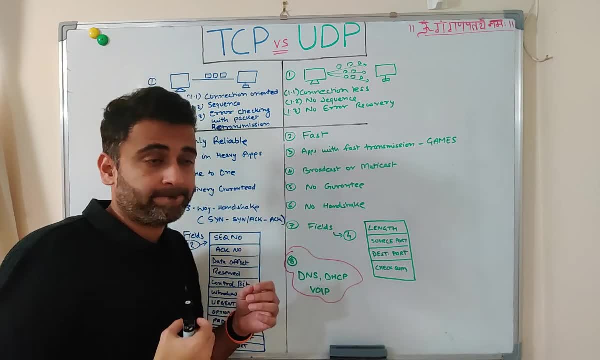 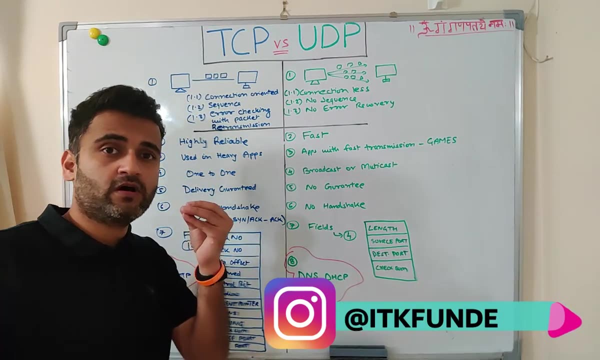 message or, for that instance, in an instagram dm. delivery is guaranteed, as i said, even if you know a packet has been sent through tcp, if, due to some reason, that particular packet is faulty or it does not work, then tcp protocol will always broadcast the message or multicast. the message, like what we do in instagram or facebook stories. we put it and we let everyone know that we have put up a story wherein, you know, tcp protocol does not reach the message like what we do in instagram or facebook stories. we put it and we let everyone know that through. tcp protocol. if you know a tcp protocol is faulty or it does not reach the message or multicast, the message or the tcp protocol will always be broadcasted so you can see that even if it is not reached, there is a loss. there is a information loss over the. 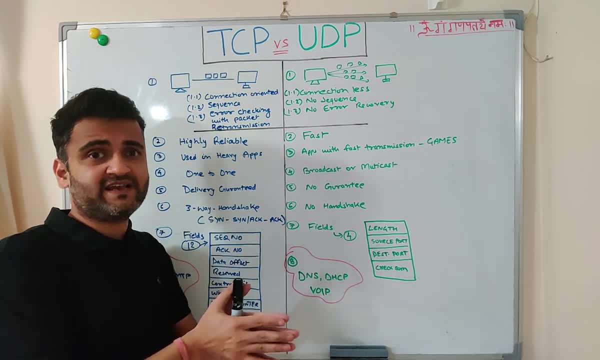 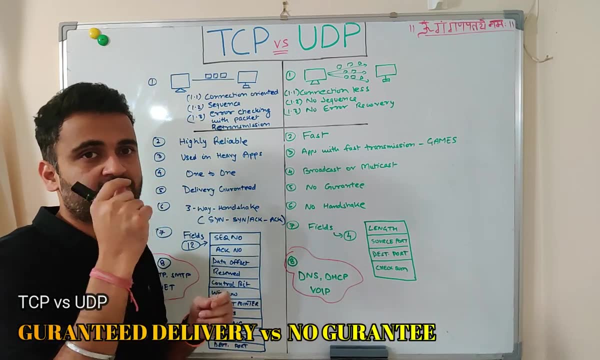 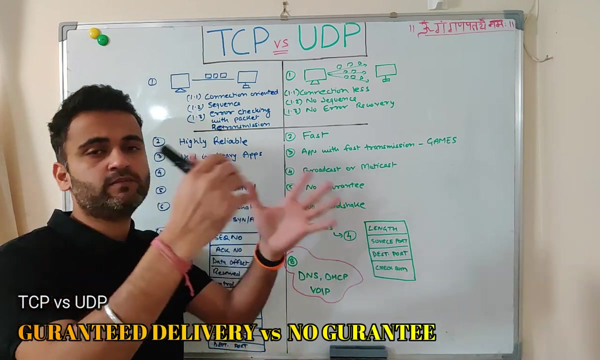 network, then it has, you know, the error checking and the sequencing in place so that it ensures that, even if it has not reached, it will again make sure that the packets are delivered, wherein here it is no guarantee, even if you know if there are 100 packets, those 100 packets will. 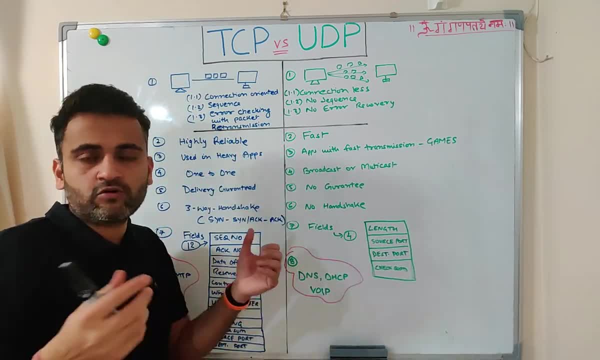 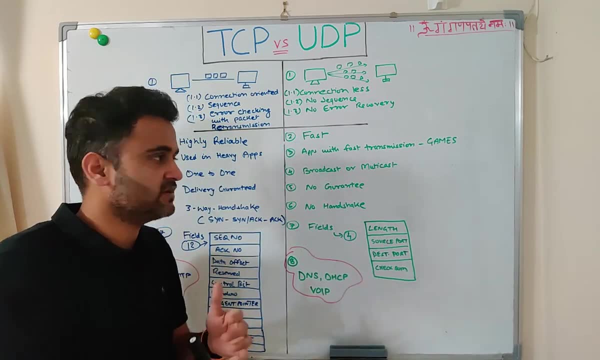 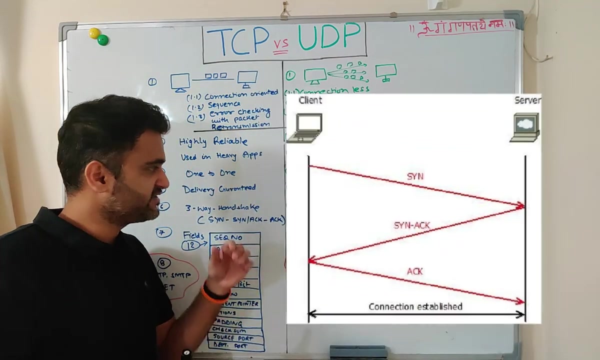 be broadcasted, maybe only 80 packets would reach the destination. 20 might be lost. this is just an example i am giving. so there is no guarantee that every packet will reach the destination. whenever tcp establishes a connection it starts with a three-way handshake. so it sends a syn packet, then it has, it gets a syn act which is syn, and 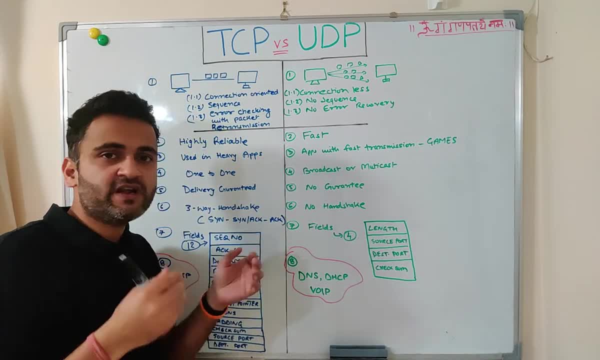 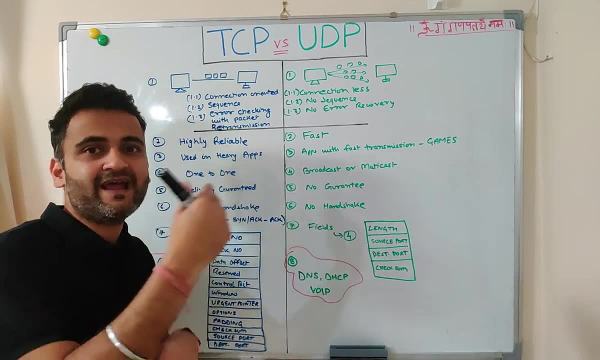 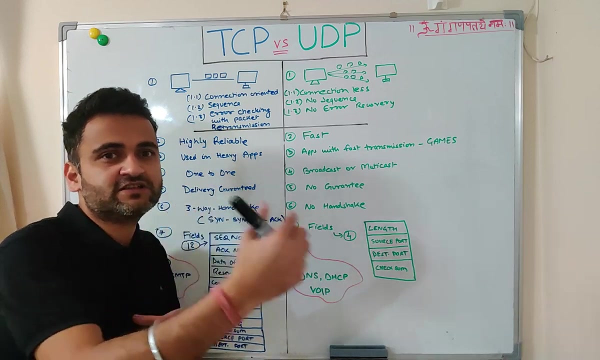 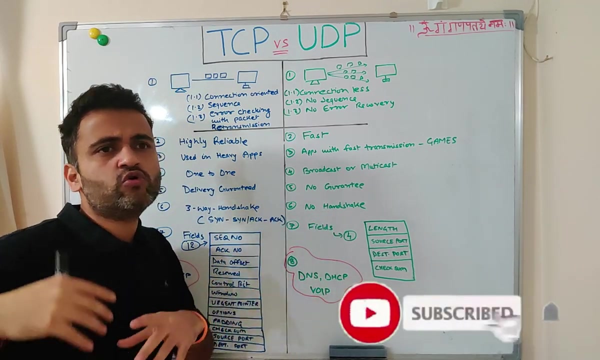 acknowledgement and then the finally act packet, which is acknowledgement. once this three-way handshake is done, then you know that communication channel is established between sender and the receiver, and that's why it becomes quite slow in nature, because you have to always rely on this three-way handshake for transferring any kind of data wherein herein, you have no handshake. you. 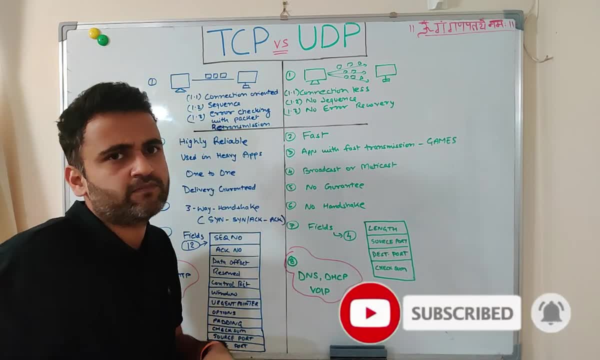 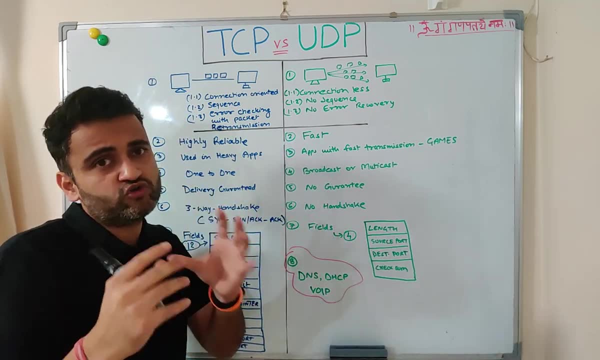 don't you know specifically send something to one specific person, you just one particular device, sorry, and you just broadcast it over the network and whosoever wants to receive it will receive it. so, when it comes to the tcpip fields, there are 12 fields in a tcp. 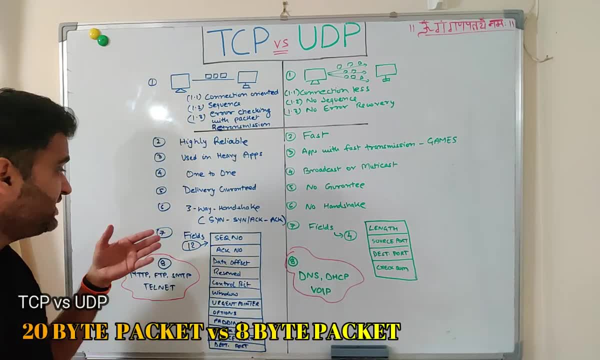 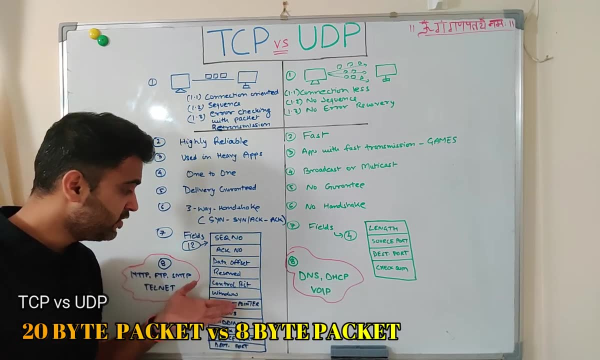 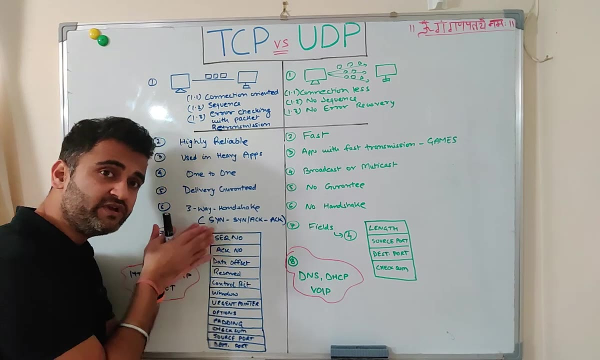 packet and there are four fields in a udp packet. in tcp packet we have these two: 12 field sequence number, acknowledgement number, data offset, reserved control bit window, urgent pointer options, padding checksum, source port and destination port. now we are not going into each and every- uh, you know each. 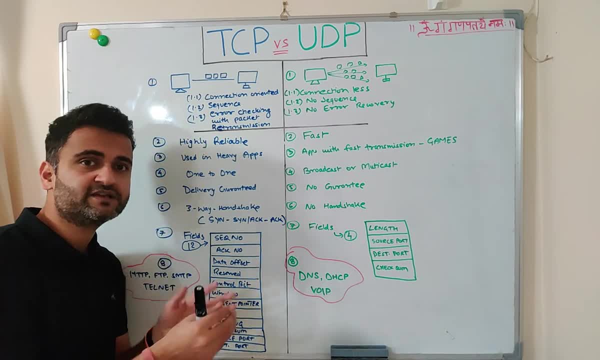 and every section and each, every field. i might give you a link in the description. you can go and check that out. you will have all the information there. and similarly, on the udp side, we have only one field in the tcp packet and there are four fields in a udp packet and there are four fields. 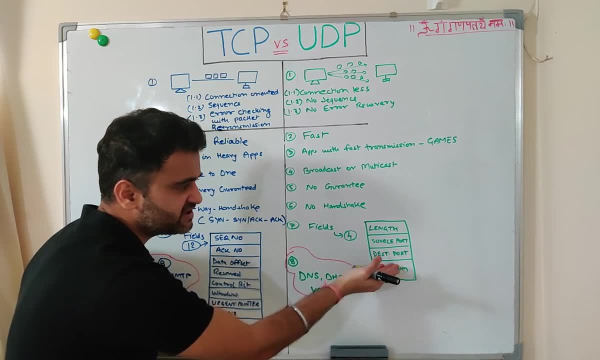 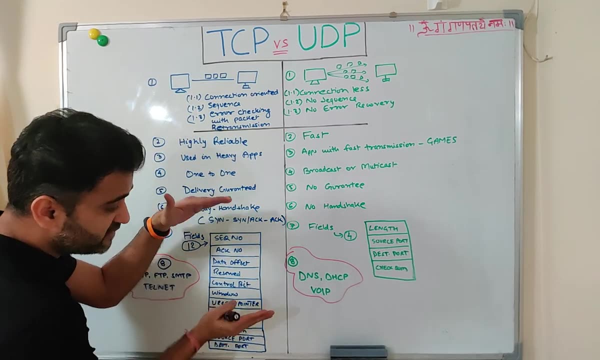 only you know four different fields: length, source, port, destination port and checksum. so by default you can see that if you are sending this much information in one packet in over the network, obviously this will be more reliable because it has more error checking and all the control fields. 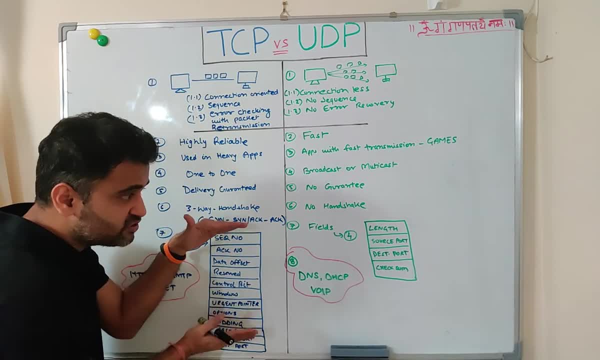 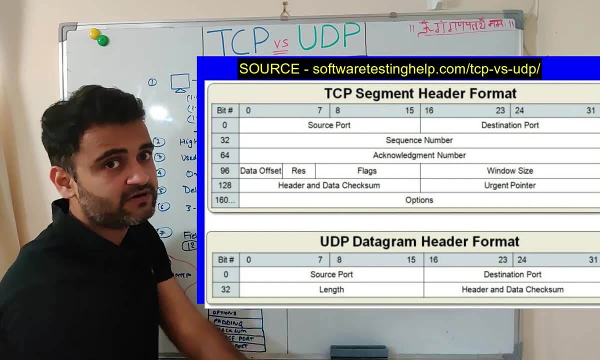 in place, but obviously it will be more heavy also to be sent, so it will be slower. herein you will have less reliability because you are not making sure that this reaches on time. but then it will be lighter and it will reach on time like it will reach faster. so now let's understand some protocols. 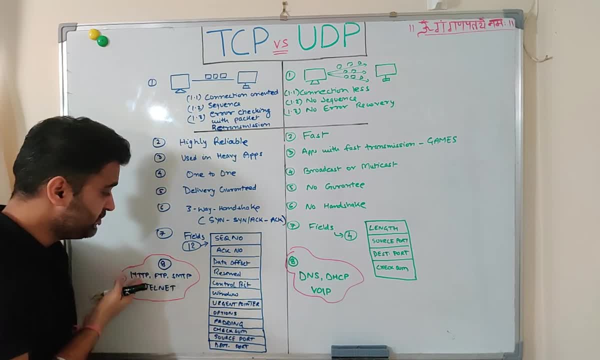 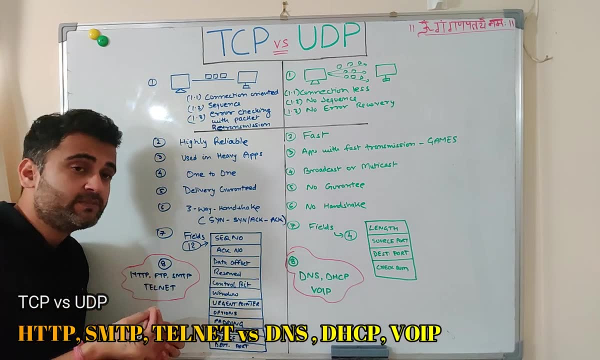 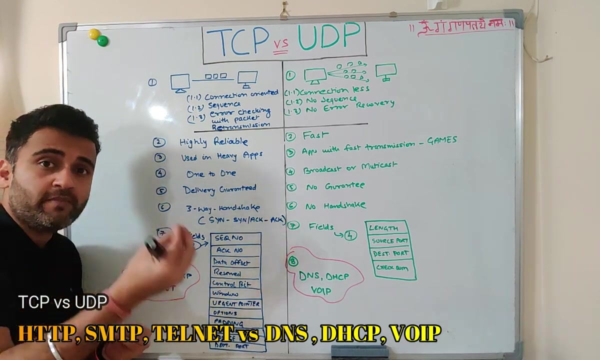 which are, which are which uses tcp protocol. so http, ftp, smtp, telnet, all these protocols are some example protocols which uses uh, the tcp protocol. http is uh used over the web, uh, ftp is your file transfer protocol. smtp is used for mail, uh mailing. telnet is again. uh is a tcp protocol. to understand. 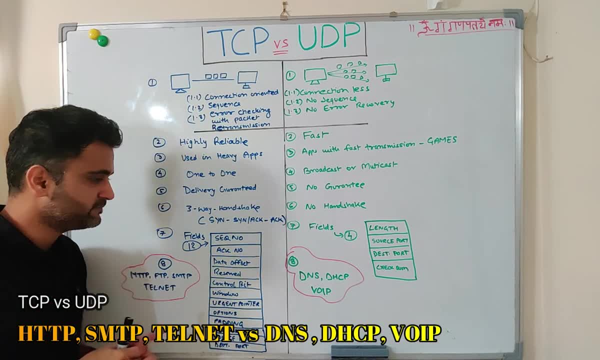 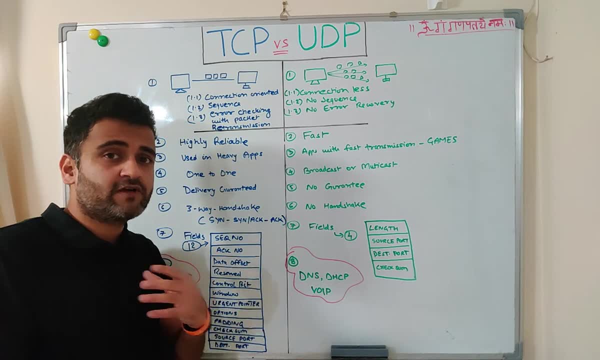 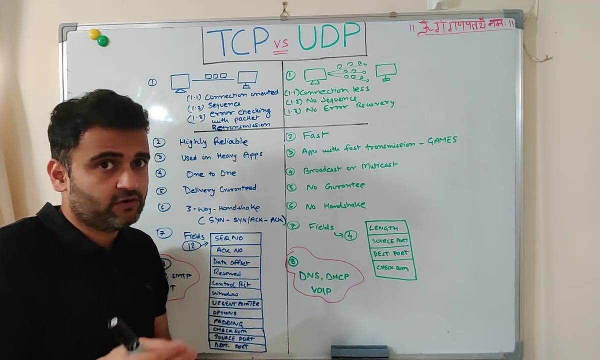 whether you are able to reach a particular device over the network on a specific port now in this utp protocol. dns: domain name server: in our next video we will be covering domain name service, so you will understand more about it. dscp we have already covered in the previous video, so if you 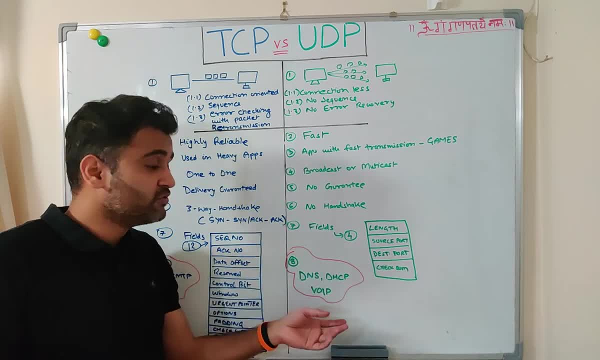 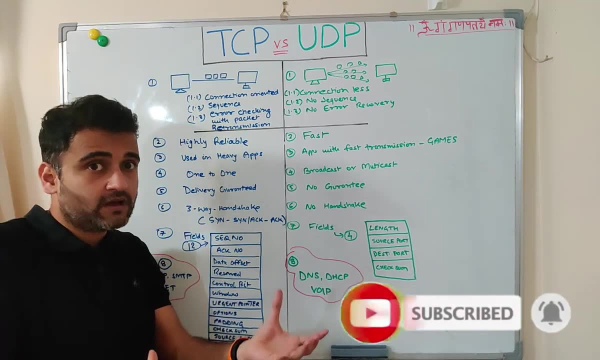 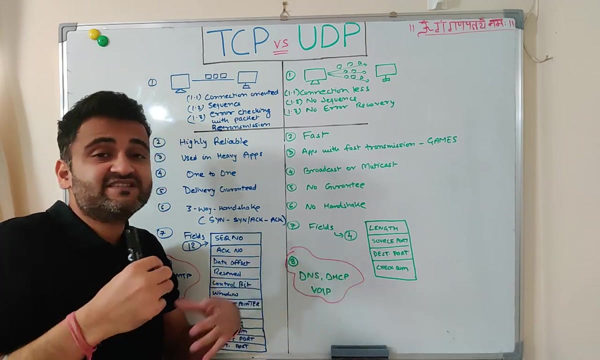 have not checked it. check that out. i have told in that video that in dscp you try to get an ip address as soon as you come into the network, and what a machine does in that. in that case it broadcasts that okay, i am in the network, i want an ip, and then whichever dscp server is there in. 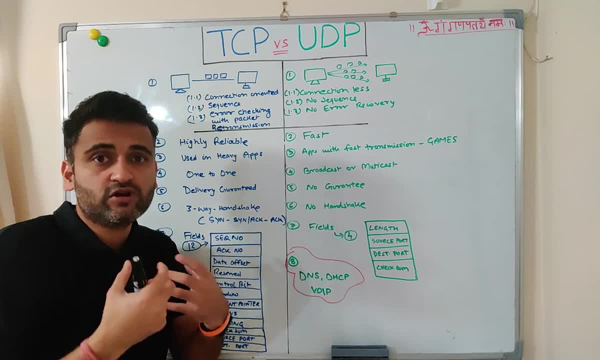 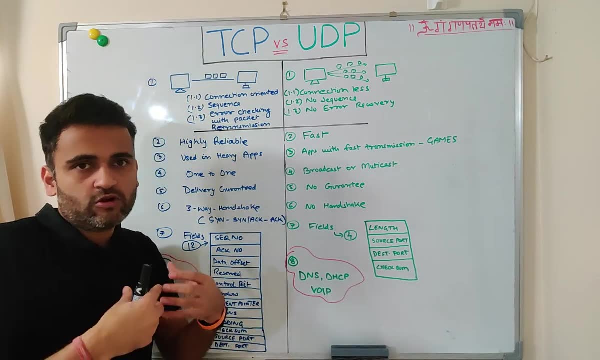 the network takes that request and assigns an ip address to that particular new device. so obviously, when you are broadcasting, obviously you are using udp protocol, voice over ip. now, these are the you know these uh. this protocol is used when you are using- uh you know- your telephones over the internet. 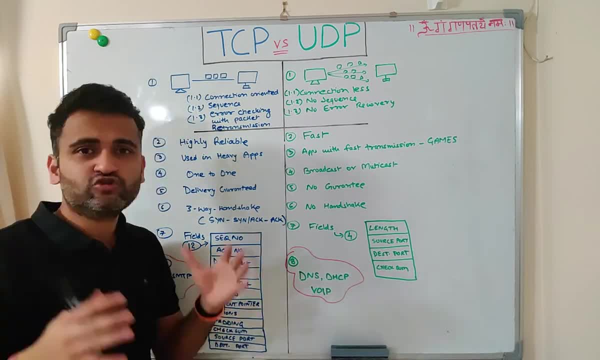 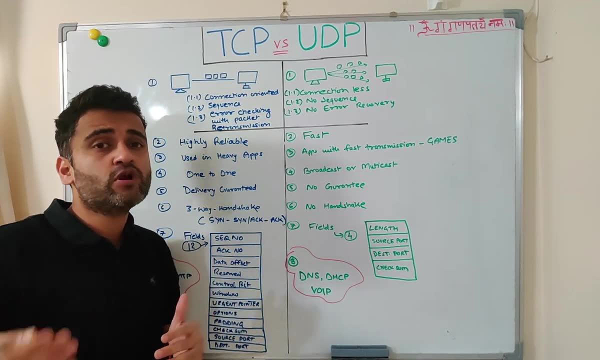 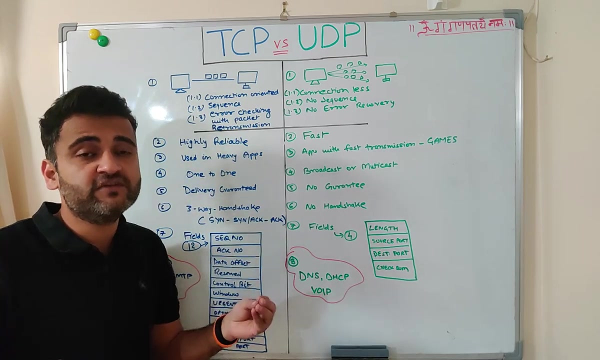 and that's why this also uses your udp protocol. so, friends, these were some very quick differences between tcp and udp protocol, and i hope now, whenever you learn more about tcp and udp, you come to know that where, uh, you know in which scenario tcp is better and in which scenarios udp.